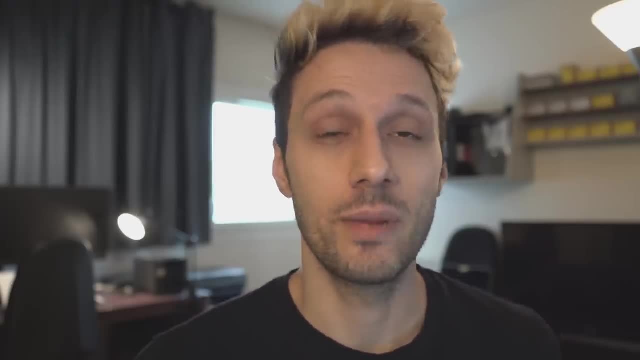 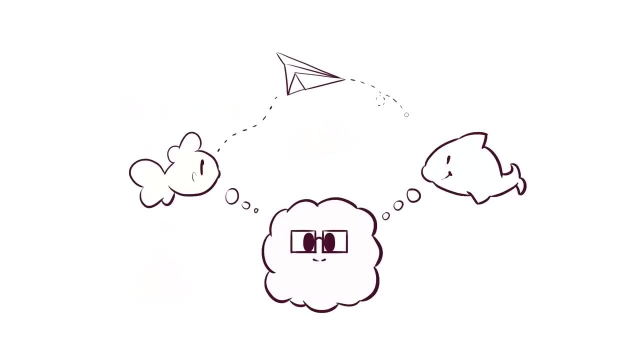 a few years back. That helps us understand that information is not learned in the same way. It's not stored in the same way. Now, this is where science comes. We have both short-term and long-term memory. Our goal is to send all what we learn to the long-term memory so that we can later retrieve it when. 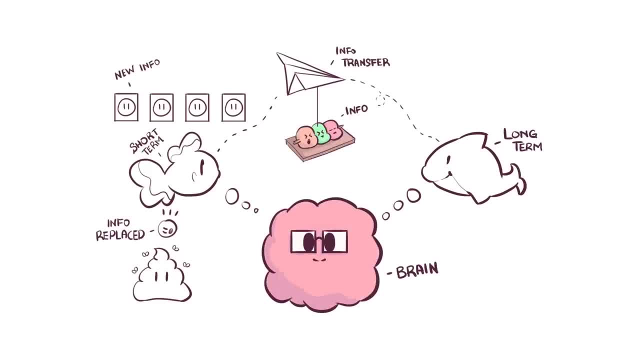 creating artwork. To put it in a simplified and fun way, think of the short-term memory as a place in the brain that has a few slots to store data with a very limited space. Whenever we learn something, the information will occupy one of these slots. Now, 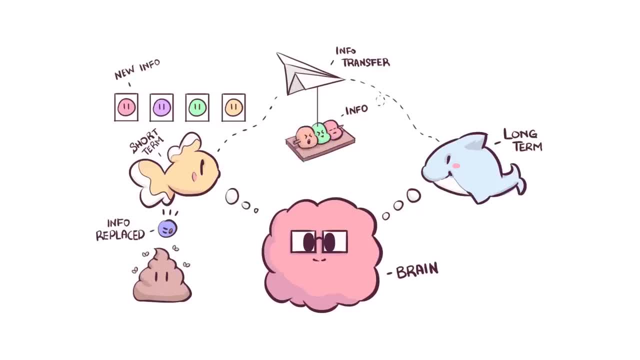 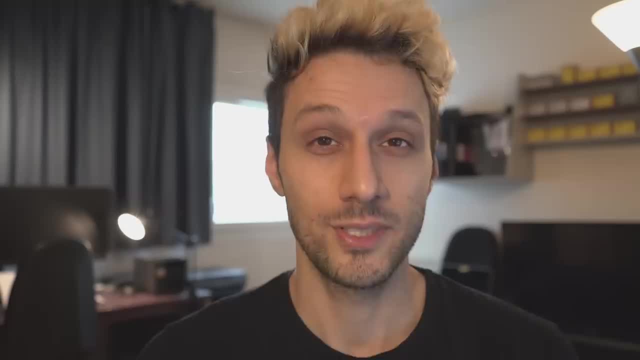 if we keep on overloading our brains with more information, the data will get dumped to be replaced by new ones, rendering our efforts in practicing inefficient, as most of it will be lost. So instead, we want to make sure that the majority of what we learn gets sent to the 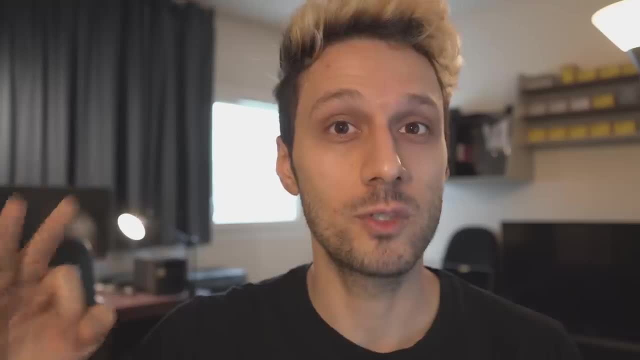 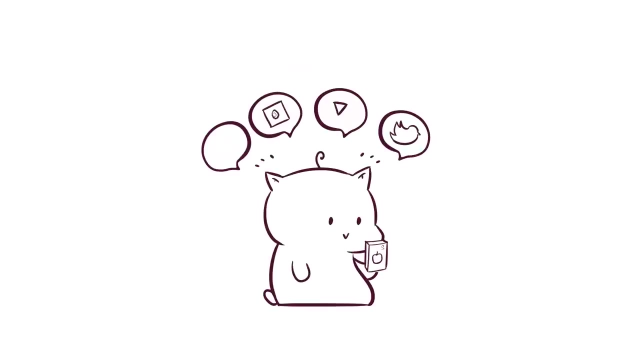 long-term memory. To do so, there are three things I want you to stop doing and five things I want you to start doing to start learning effectively. The first thing is getting rid of all of distractions and overloading of information when you are practicing and learning art-related stuff. 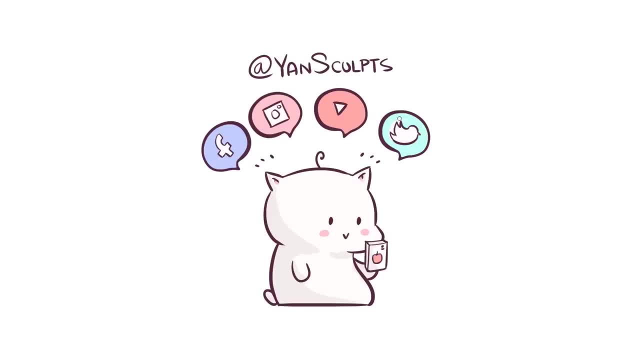 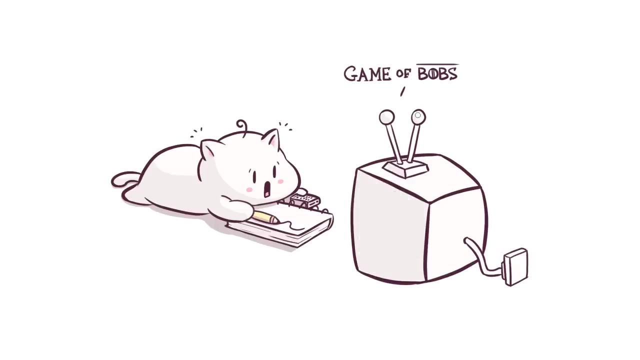 So no more checking your phone, Facebook, Instagram. You get the point. The sole focus during a study session should be practicing art and nothing else. The second thing is to completely stop multitasking, as there is research that shows that daily multitaskers are easily distracted and suffer from a poor attention span. 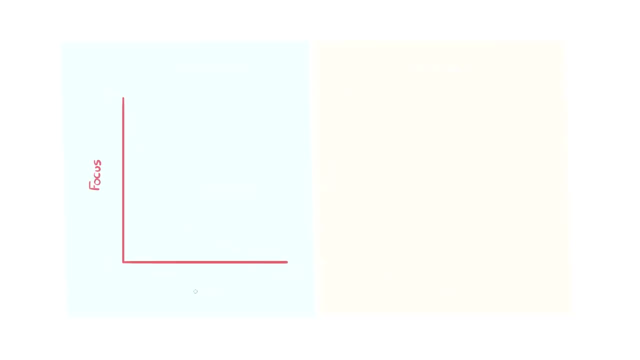 hence being less productive and inefficient. The third thing is to stop practicing for long sessions without taking breaks in between. There have been estimates that, on average, the attention span of adults lasts between 10 to 20 minutes before it starts diminishing, which is insane. So taking a 2 to 5 minute break every 20 to 30. 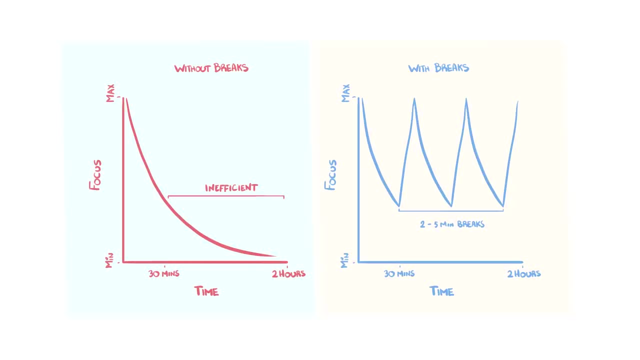 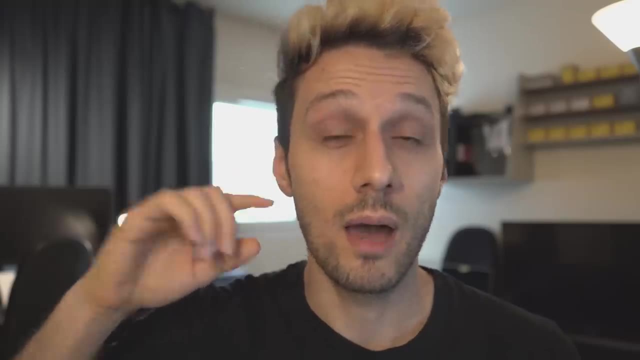 minutes will jumpstart your focus, allowing you to benefit from longer hours of practice. Okay, let's start talking about some effective methods to commit information you learn to your long-term memory. I want you to start doing these five things: Deconstruction, recall. 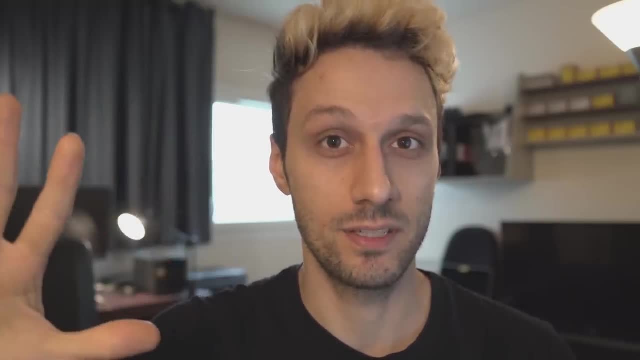 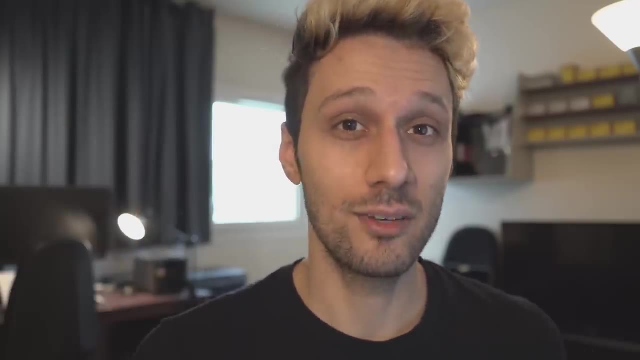 self-critique, quality sleep and spaced repetition. To go over these five methods, let me use the example I gave you on Bob, who got to level 10 after one year of practicing art, and Dave, who got to level 50 in that same amount of time. So I'm going to explain how each of them 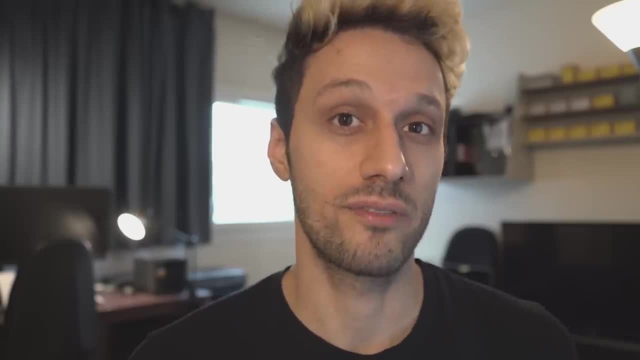 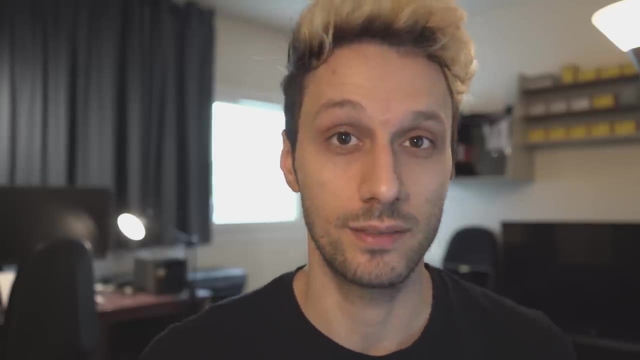 works differently. For this example, Bob and Dave are both trying to learn how to draw faces. However, whatever I'm going to teach you right now will apply to anything else, including any other art medium, such as sculpting. Bob spent every day drawing different faces, using 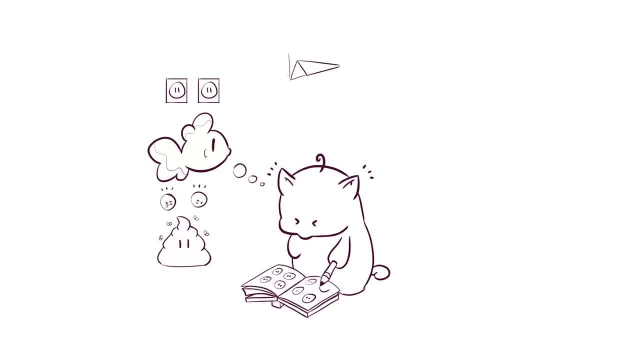 reference from Pinterest. He would look at the reference and draw what he sees, no more and no less. He kept drawing a bunch of different heads per day, and every one he does occupies one of his short-term memory slots. Since Bob here has two of these slots, he constantly replaces what he learns with new. 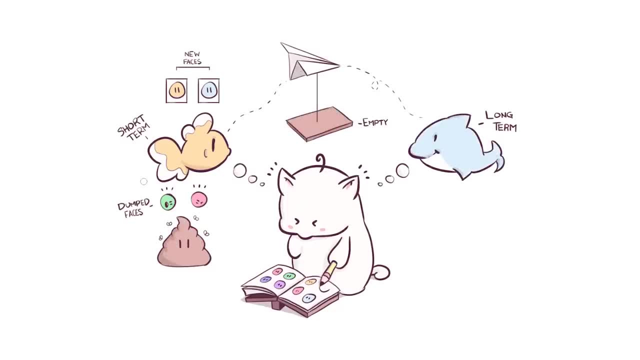 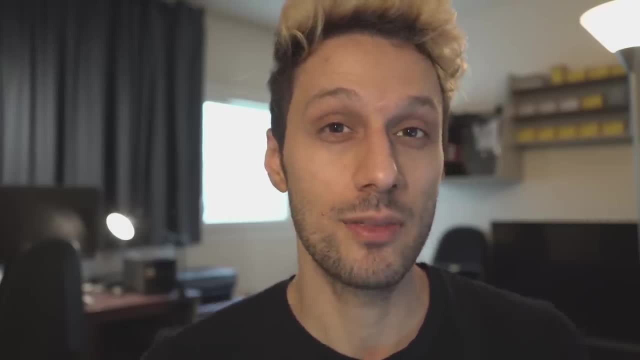 information without even noticing it. So let's get started. This, again, is a very simplified way used to illustrate my point. That said, we can quickly see how this method is just not efficient. Most of what we're learning is getting mixed and lost, slowing down our growth as artists. So let's take Dave, Dave. 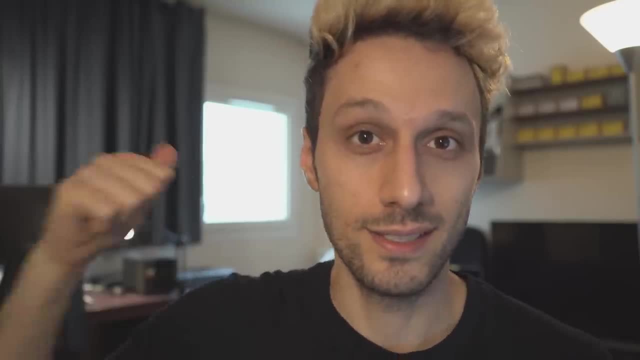 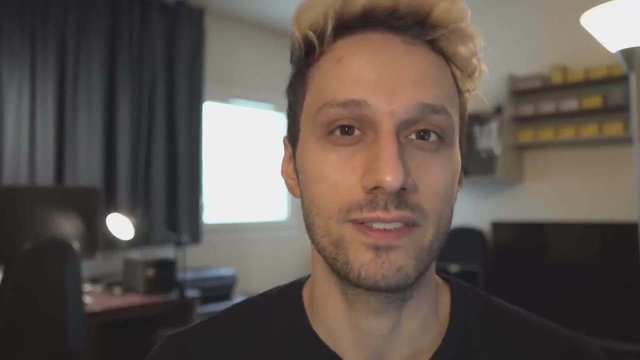 was smart enough to follow the five steps I just talked about: Deconstruction, recall, self-critique, quality sleep and spaced repetition. Let's see how he applied all of these five steps. Like Bob, Dave also drew a lot of faces. He, however, doesn't only rely on reference. He also. 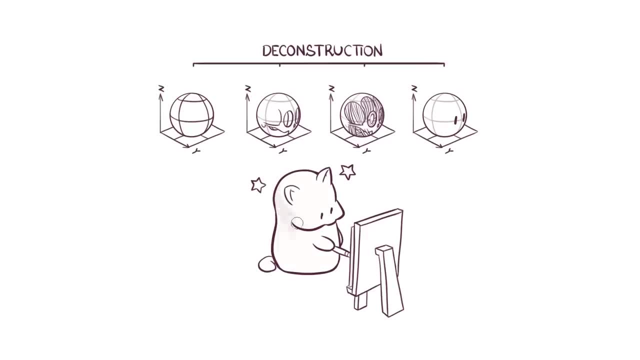 consciously deconstructs what he sees, either visually or on paper. This is to say that he is truly putting in the effort in learning how things actually work. For example, he tries to figure out the perspective of that head, how the head would be in geometric, simple shapes. 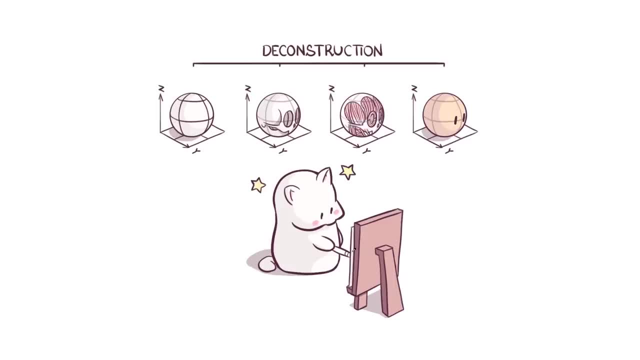 how the skull underneath would look like the muscles, their names, their functions, etc. Dave then repeats the same head drawing without looking at reference to his best ability to remember what he just drew. This is called recall. He will then do some self-critique. 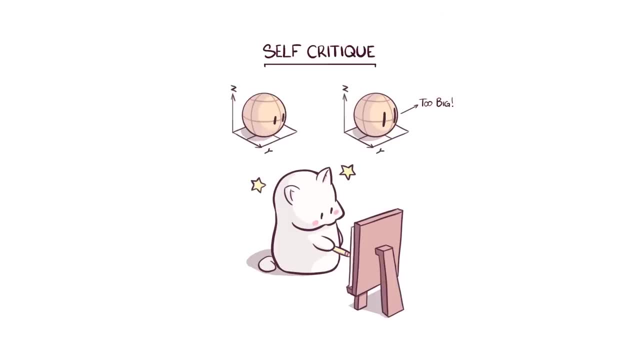 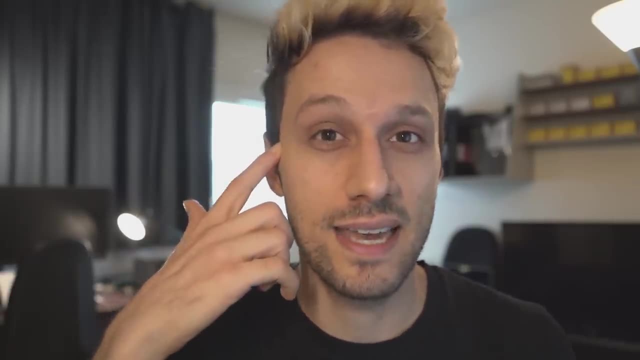 by comparing differences between his drawings and the reference to figure out what he forgot or did wrong. This, right here, is a very powerful way to practice, as truly understanding the subject at hand, repeating it through recall, then doing some self-critique, will create a lot. 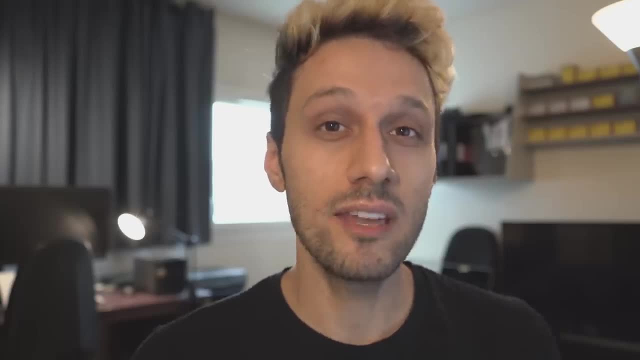 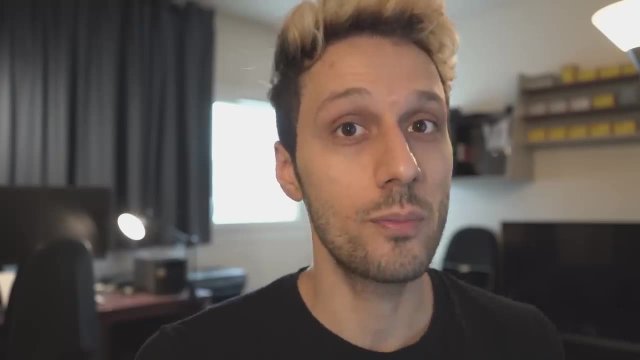 more impact to the information you're learning. By going through these steps, Dave is ensuring that whatever he practices is sustained for a longer period of time by sending the information from his short-term memory to his long-term memory before it gets replaced by any. 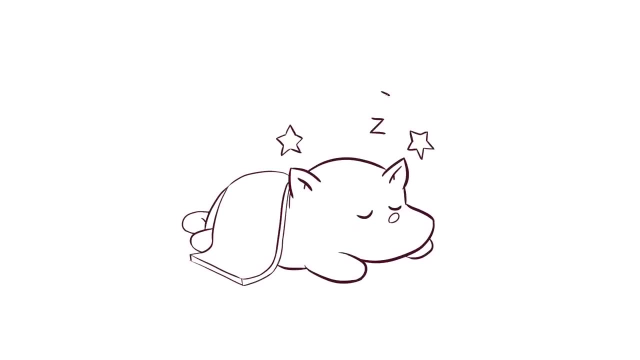 other information. After a hard day of practice using these three steps for whatever he draws, he will get a good night's sleep, which will help him properly retain any information he acquired. This now takes us to the last step: spaced repetition. You need to see the brain as a 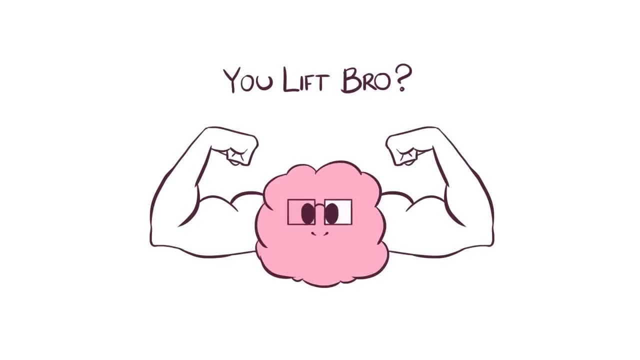 muscle. it needs maintenance. Repeating what you learned over and over again throughout the month and year will reinforce the information, help you better understand it and also make it last for a longer period of time. This is a very important step to take into account when you're learning. 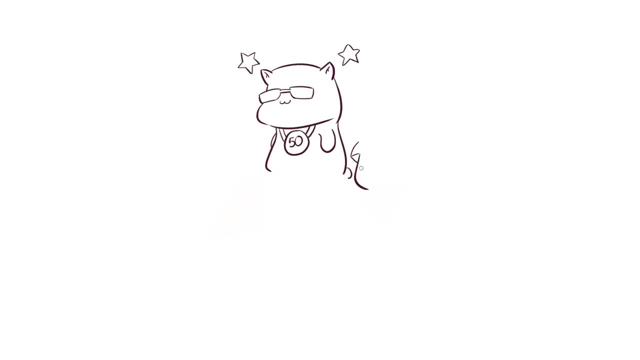 about drawing heads. So Bob here, even after one year of drawing heads, still doesn't truly understand how to draw one. Dave, on the other hand, has a very good understanding of heads. he can now draw them better than Bob, both from reference and from imagination. And now Dave is. 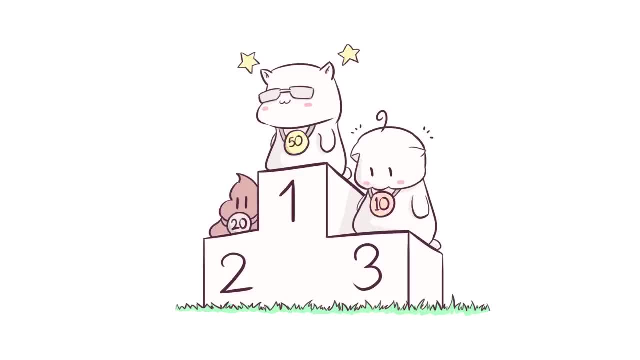 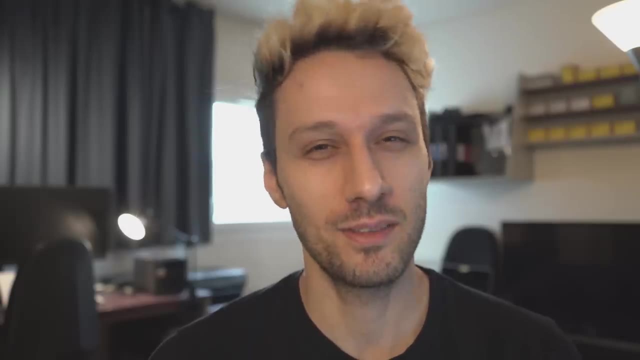 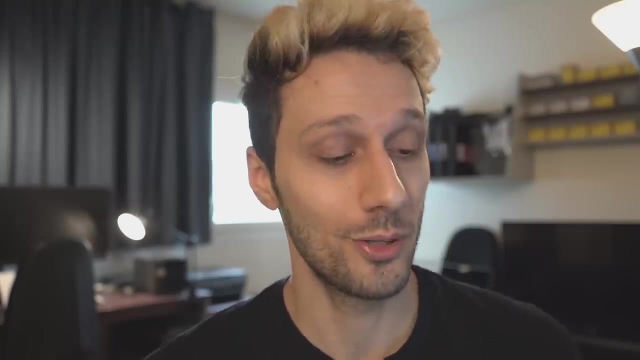 40 levels ahead of Bob. Sorry, Bob, you didn't lack talent, you simply needed to watch this video. If you liked this video, please subscribe to the channel, not the video. Give the video a like, though, and make sure to share it with your friends so that you can help this channel out. 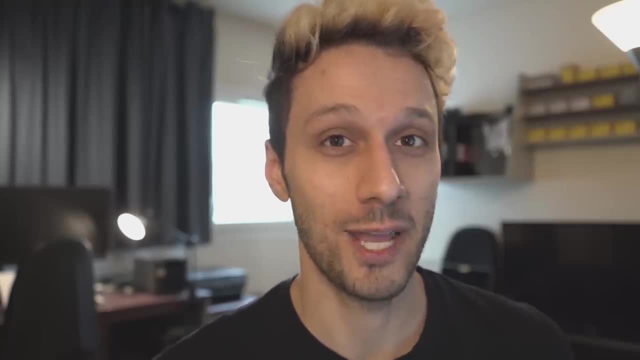 And, before you go, know that the science that I talked about over here is a lot more complicated than reality. I just wanted to simplify things in a fun way for you guys to easily retain the information and then apply it to your daily practice routine, with whatever kind of art you 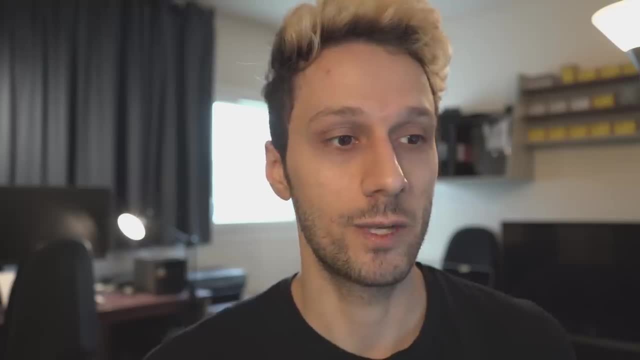 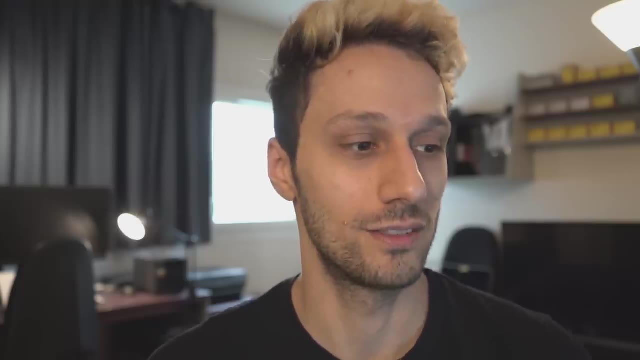 create. So there are still a lot of things I can cover and a lot of different methods that we can learn from science to improve our art, And I've been really interested in the subject lately, you know, with psychology and how the brain works and all of that. So if you're interested in that, 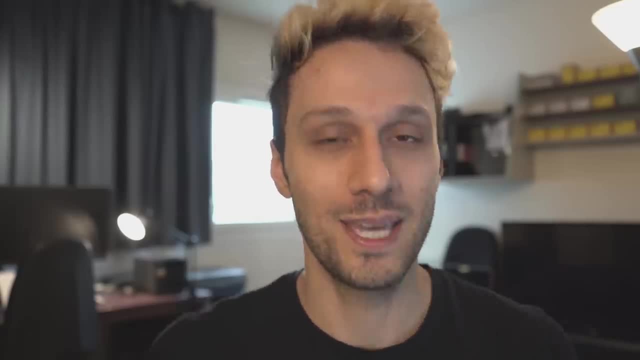 kind of stuff. if this video helped you out and you really enjoyed it, just make sure that you let me know in the comment section below so that I can create more of this type of video. Anyways, I'll see you guys in the next one, So let me ask you, okay. 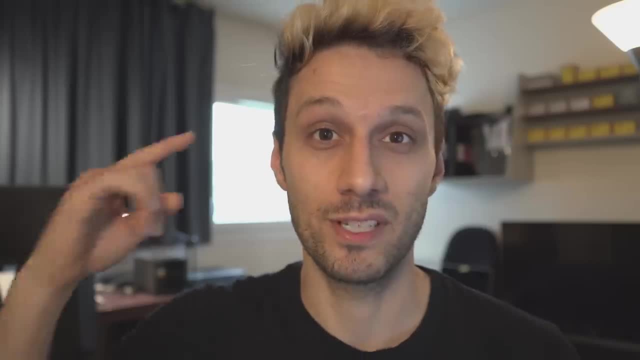 okay, let's start talking about some effective methods to commit information you learn to your life. So let me ask you, okay, let's start talking about some effective methods to commit long-term memory- Are you a Bob or are you Dave- How the brain works, all that kind of stuff.